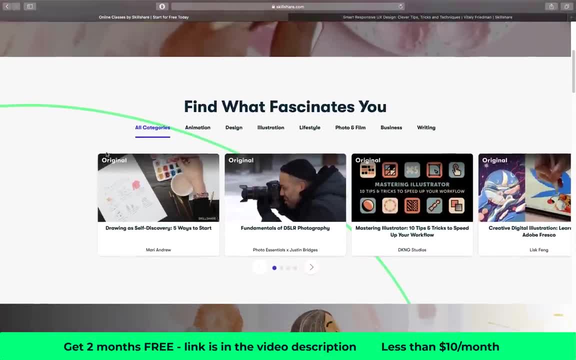 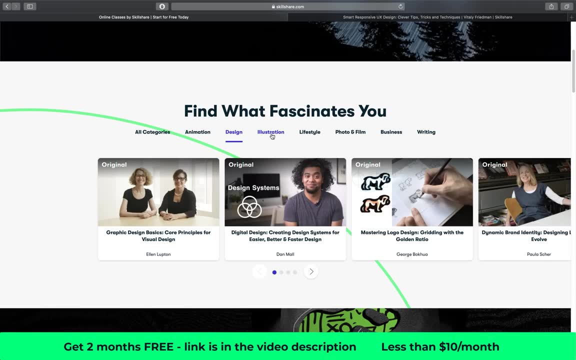 video and supporting OneSkillz channel. Skillshare is an awesome online learning community with thousands of classes for you, my friend. You can learn many new skills, such as animation, design and illustration and many more, And I hope you enjoy this tutorial and I will see you in the next one. 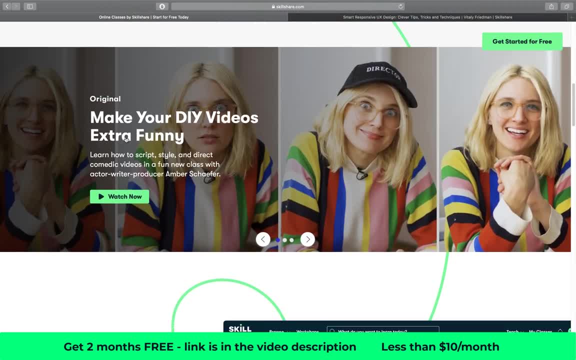 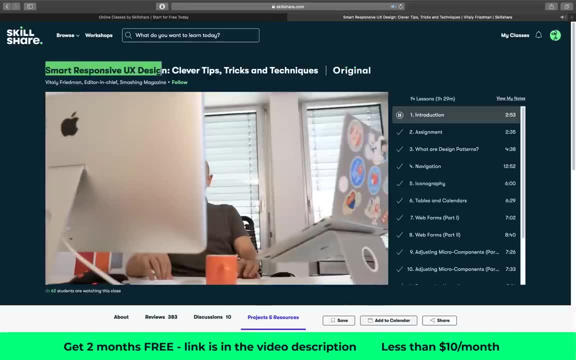 I am always looking for new ways to improve myself as a presentation designer, and learning new skills such as user experience design is really useful. I have recently taken this class on Skillshare called Smart, Responsive UX Design – Clever Tips, Tricks and Techniques by Vitaly from Smashing. 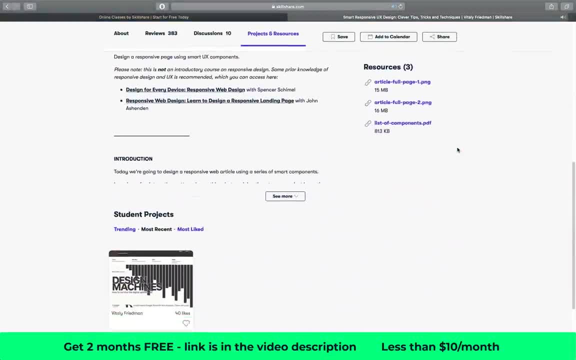 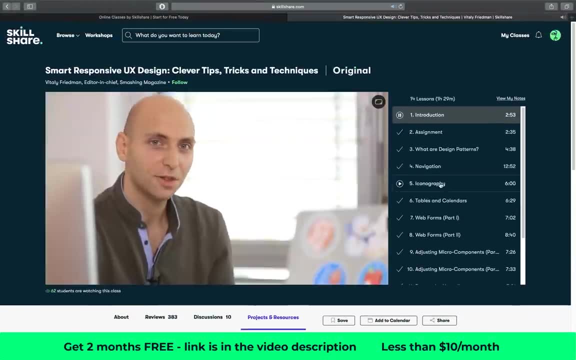 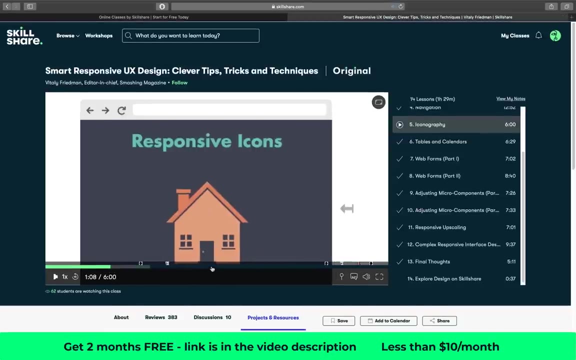 Magazine, And this class was all about making a better responsive website experience for your web visitors. However, I think many of the principles can be applied to slide design as well, And in today's video, we will be doing our best to create a nice user experience with our animated PowerPoint. 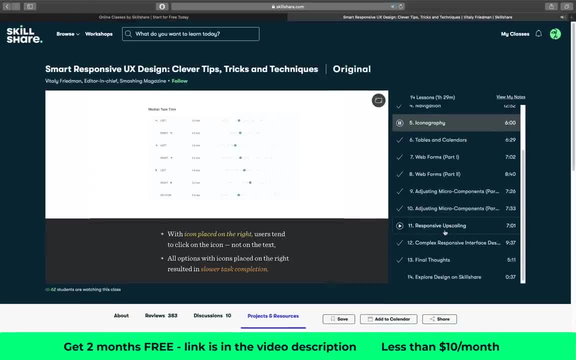 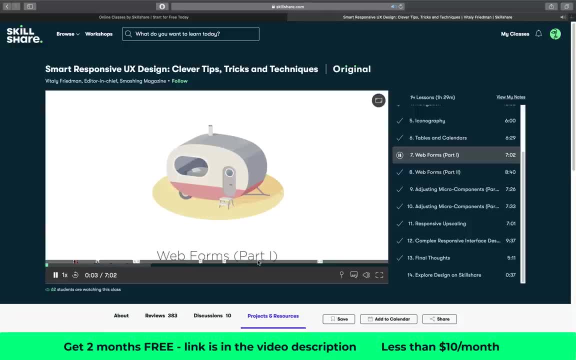 slide design. So definitely check out Skillshare and start creating even more amazing presentations. First 1000 people who click the link in the video description will get 2 months of Skillshare Premium for free. And, by the way, today's tutorial slides are free to download, thanks to Skillshare. 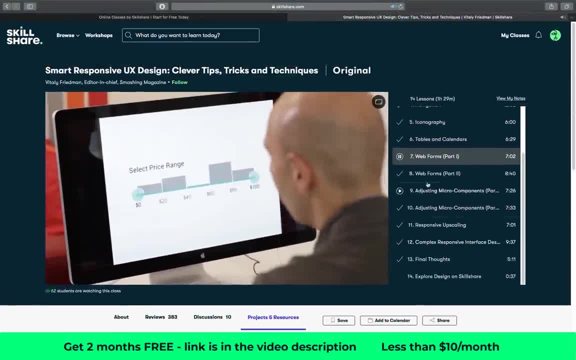 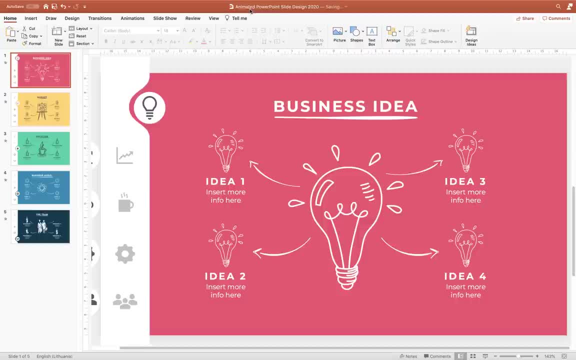 Link is in the video description. And now let's continue with the video. So, ladies and gentlemen, I hope you enjoyed this video. If you liked it, give it a thumbs up and let me show you how you can create this amazing animated PowerPoint slide design. So, first of all, 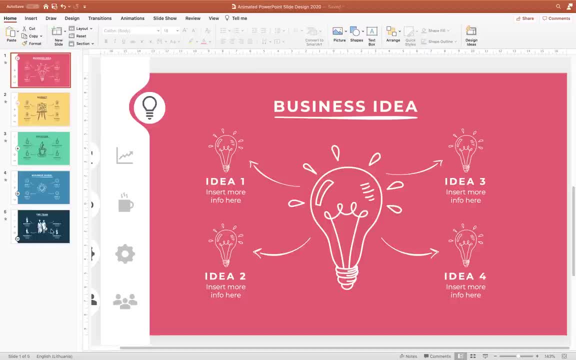 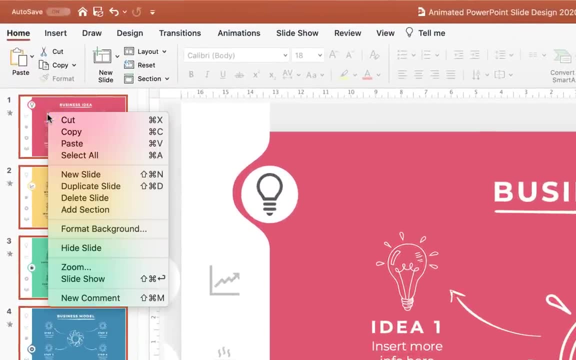 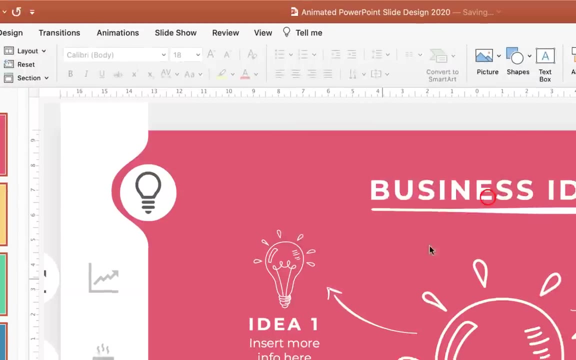 let me just choose, while holding down the shift key, all of these slides, all of these five slides that I have already created, And let's just add them to a slide section. Let's call it original. And here below, let's start a new section And let's call it. 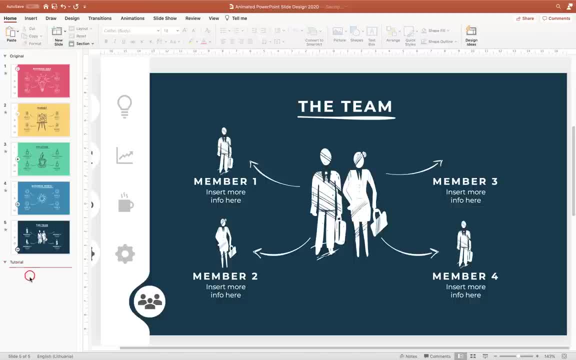 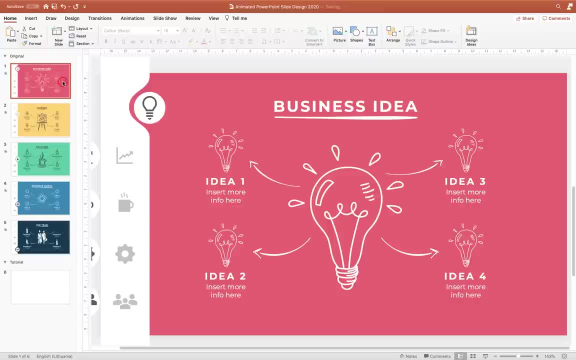 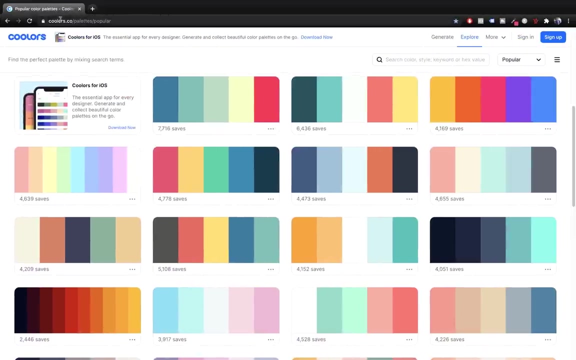 Tutorial: Alright, and here let's add a new slide, Alright. so first of all, let's take care of the color palette. So, as you can see, here we have five different slides with five beautiful background colors, So you can always go to Coolersco or colorsco and find beautiful palettes. 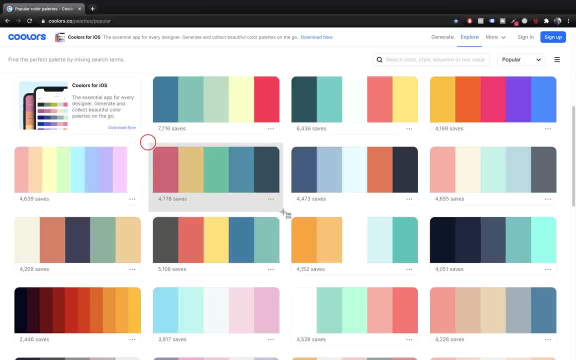 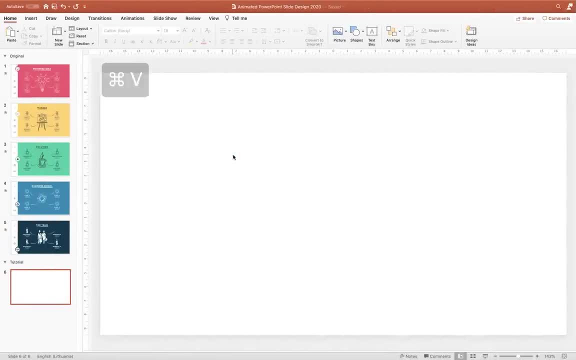 So let's just grab Colorsco, if you are familiar with colorsco. So now I want to add two colors, So this beautiful color palette. so i'm just using a screen capture tool and let's just hit command v or control v to paste this palette right here. all right, let's zoom out a little bit, all right. 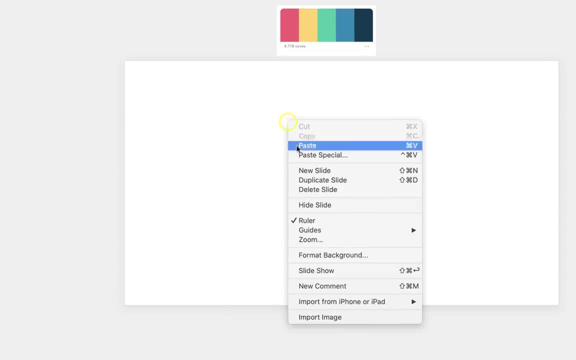 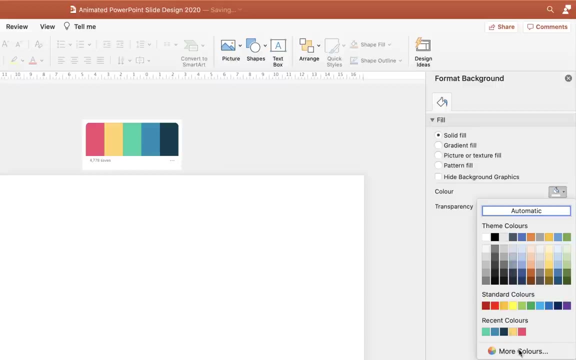 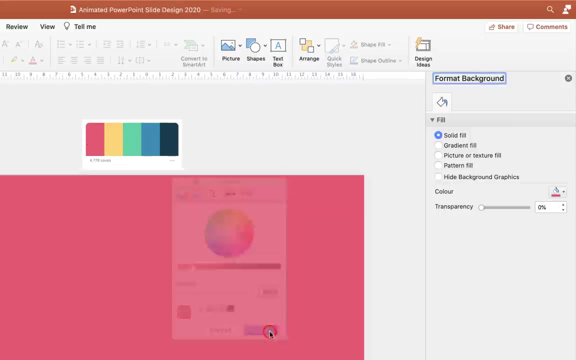 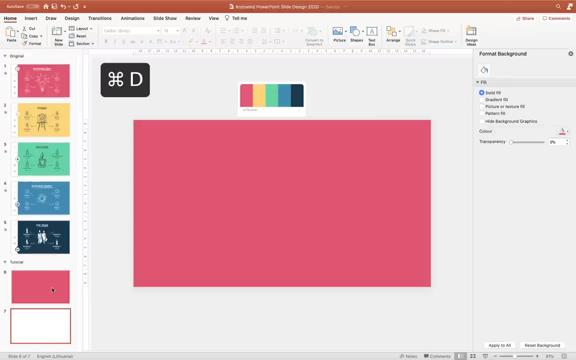 and now we can just right click on this slide, number six. choose format background. choose solid color. now let's expand the color window- more colors- and let's just use this eyedropper tool to pick this exact color. that's awesome, all right. so let me just duplicate this slide five times: one, two. 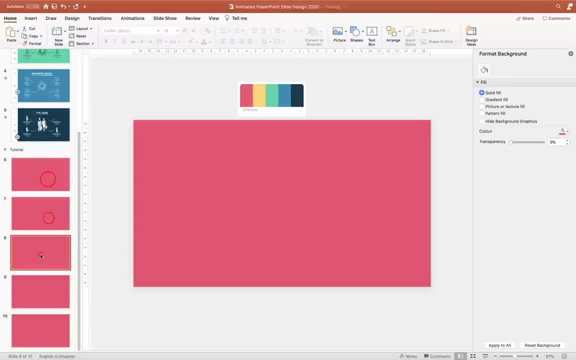 three, four, two, three, four, five, yeah, so i guess four times. now let's just change the rest of these slides, i mean the colors of the rest of these slides. so for slide number seven, let's choose this beautiful yellow color. all right, so for now i'm just choosing, choosing, choosing different colors from the color palette. 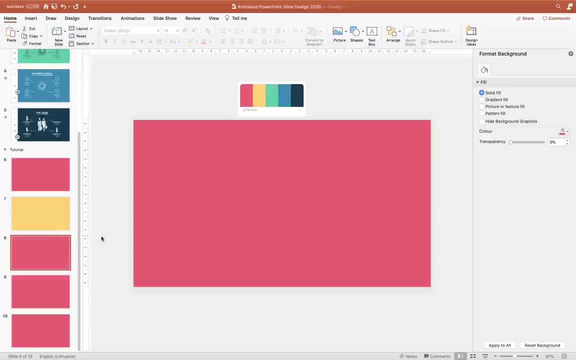 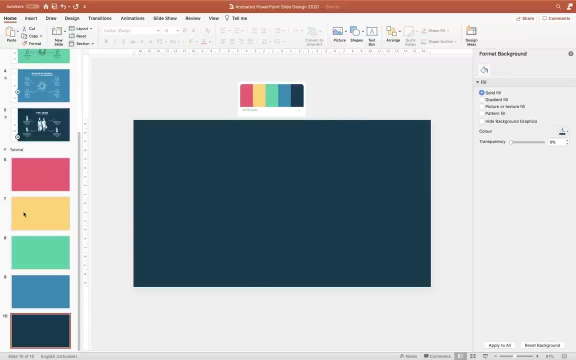 so it's pretty easy. so i'll just speed it up a little bit and i'll meet you in a second. all right, ladies and gentlemen. so now we have five new beautiful slides with a beautiful background color from our color palette, so we can delete this color palette picture. 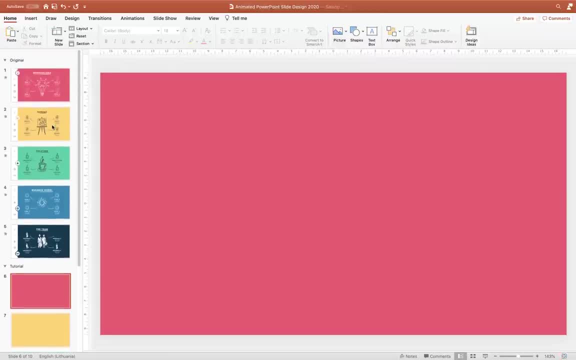 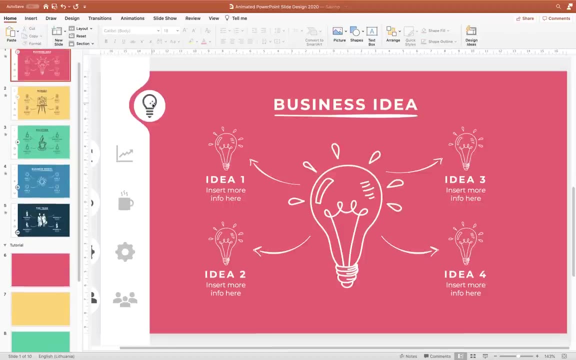 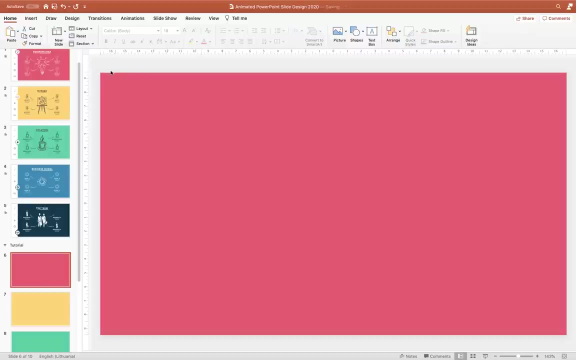 all right, let's zoom in a little bit, and now we can create these beautiful icon bubbles. uh, so first of all, we need to find the five icons so you can go to websites such as flag icon dot com. but for this tutorial, let's just use powerpoint icons if you have powerpoint office. 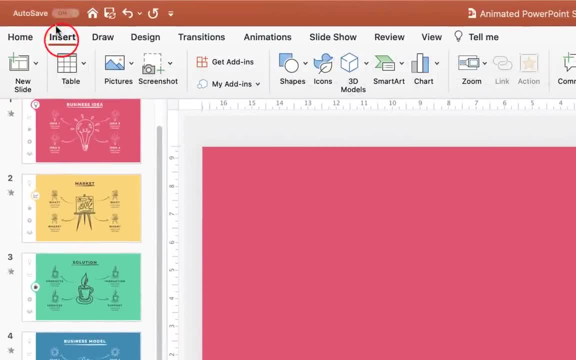 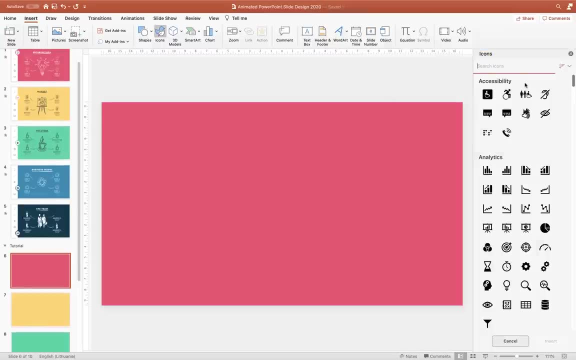 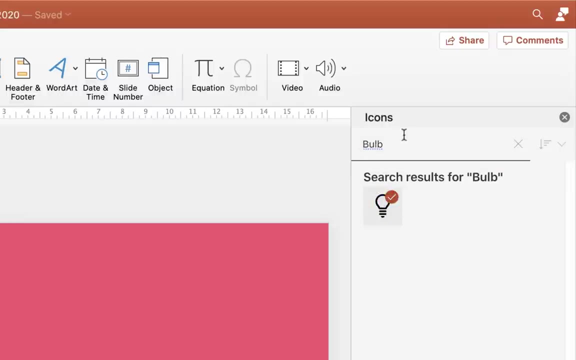 365. you should see in the insert section this icon tab, so let's just click on it. and we need to find five beautiful icons. so first of all, let's just look for bulb icon, so let's click on it to select it all. right now let's see what. 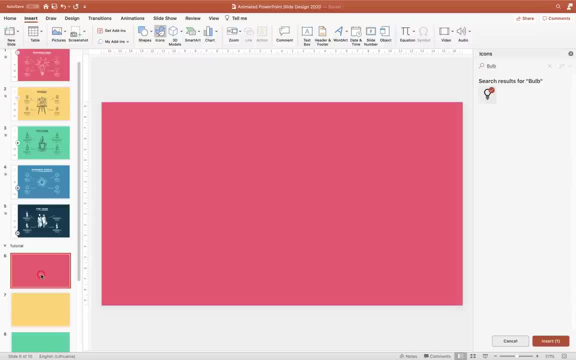 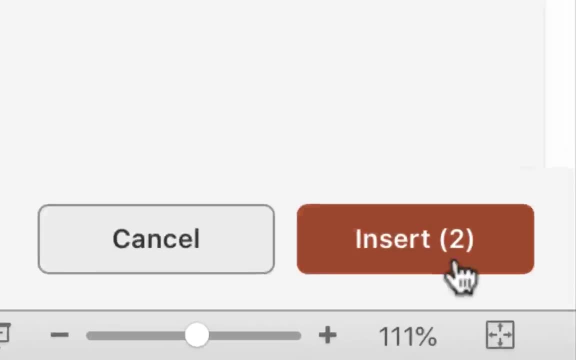 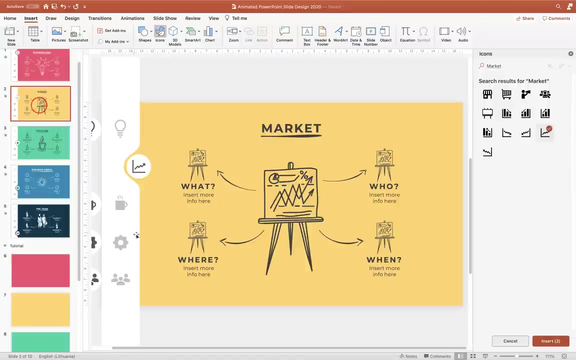 kind of other icons do we need? so let's search for market icon, let's click on this one, so, as you can see, we have insert two. so we have already two icons selected, all right, the next one is cup gear and some people, so let's find those icons. 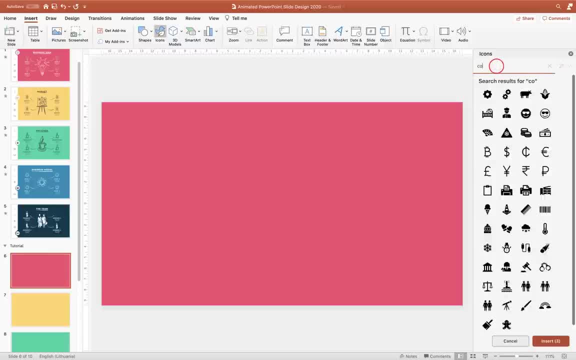 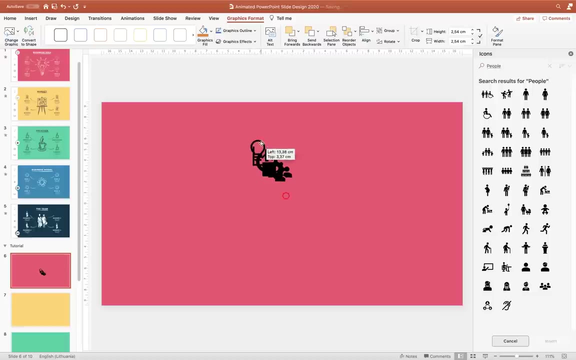 i guess i'll just type in coffee, all right here. and people, i think this one. so let's just click insert six. so i think i have accidentally selected one more icon that i don't need. so let's see, yes, i guess this one. we can delete this one, all right. 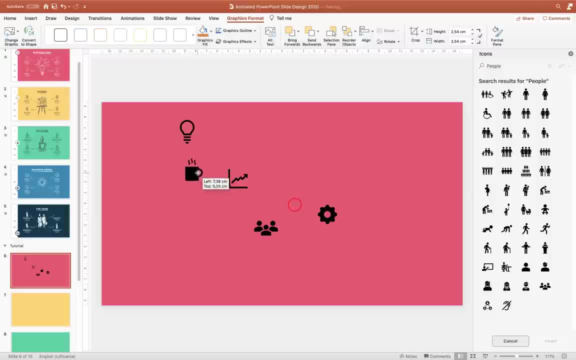 okay. so now we have all of our icons. let's align them just like this. so the next one should be market icon, then the solution, coffee cup, then the gear, and then we have some people. all right, so now let's insert a circle. so let's just go to insert shapes, let's choose circle. 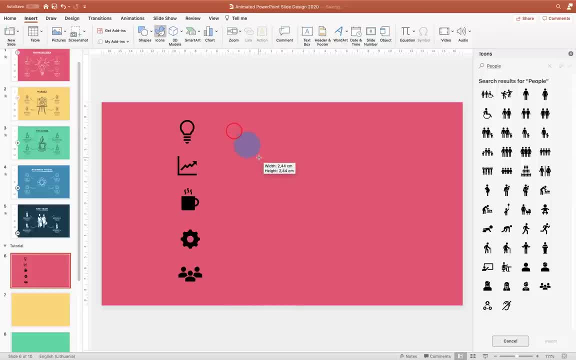 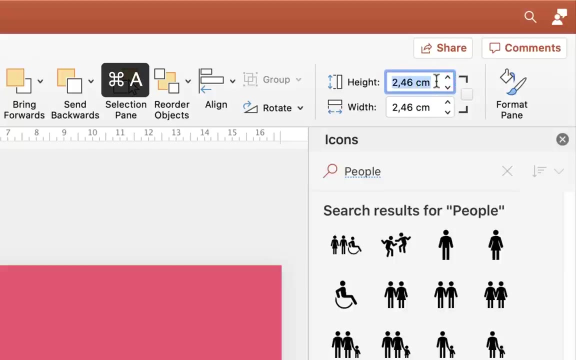 tool. hold down the shift key to get a perfect circle. all right, we can make it absolutely white, no outline- all right, and let's just place it somewhere around here. and for the size, we can actually use 2.3 centimeters. let's make sure that we. 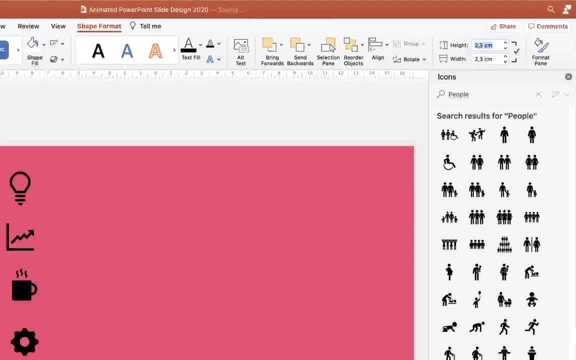 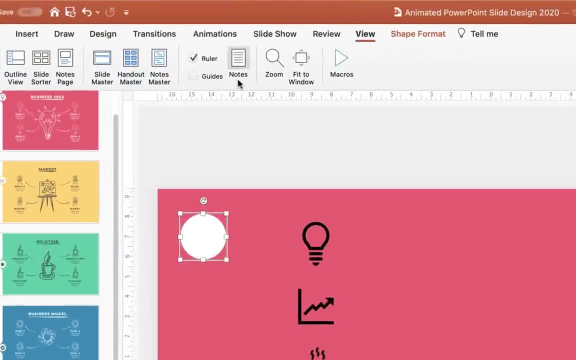 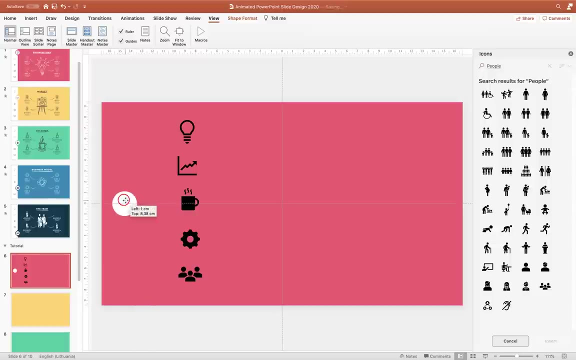 lock the aspect ratio, let's hit enter- i think 2.3 works well in this situation- and let's just activate slide guides so that we can see where is the center of the slide. so let's actually put this one in the center center of the slide, all right, just like this. and now hold down the alt or option key and drag. 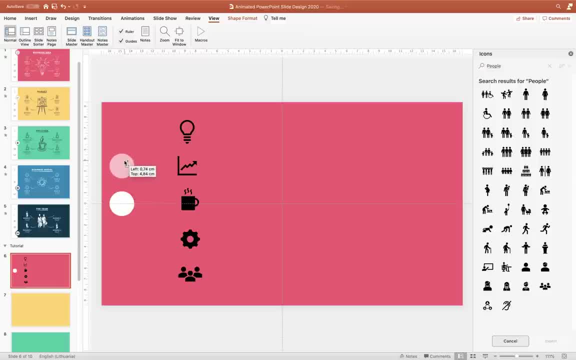 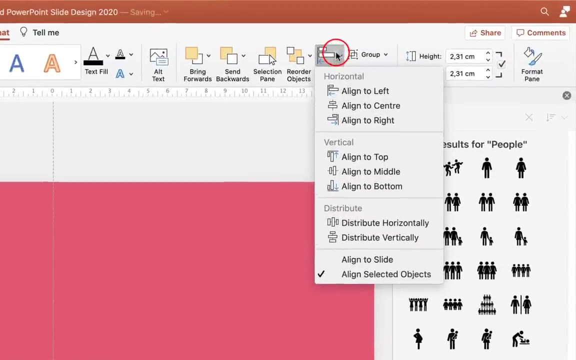 upwards so that we can make a copy. you can hold down the shift key as well to drag a copy in a straight line, just like this. all right, now we can hold down the shift key and select these three bubbles and let's make sure that we have equal vertical gaps, just like that. and now let's. 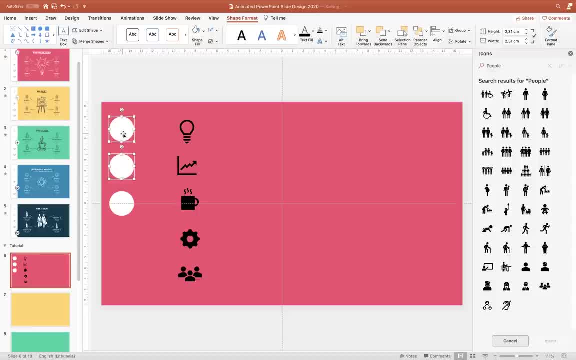 just hold down the shift key, select these two top bubbles, hold down the option or alt key and let's drag some copies below, and powerpoint should help us to align everything. perfectly awesome, and now let's make sure that we select all of our icons. let's make sure. 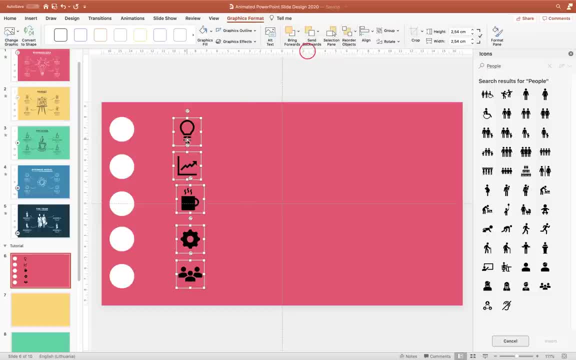 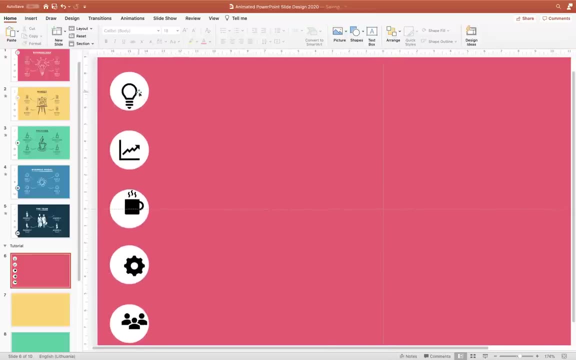 they're in the front, and now all we have to do is just fit them inside of these bubbles. so let's make all of our icons smaller, just like that. and now we can, we can zoom in and let's make sure that we fit all of these icons, one by one, into these circles. let's make this coffee cup. 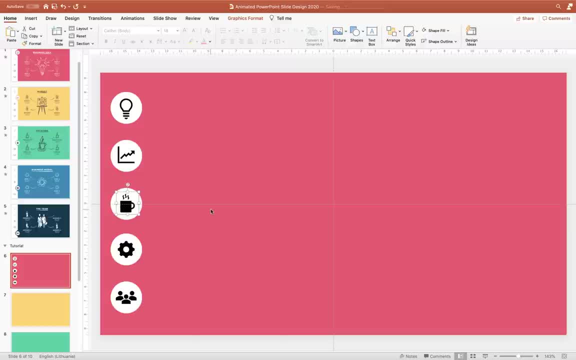 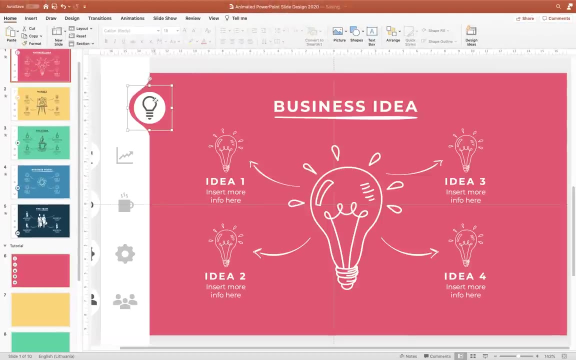 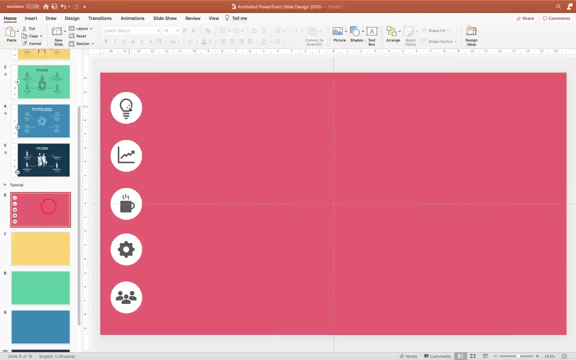 a little bit smaller, just like that, and now we can select all of the icons and let's choose its slightly different color, for example this one. let me actually check what kind of color i was using right here. yes, the second black color from the top in the second row, the second column. 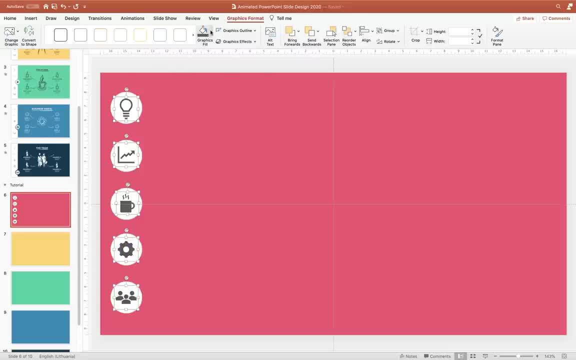 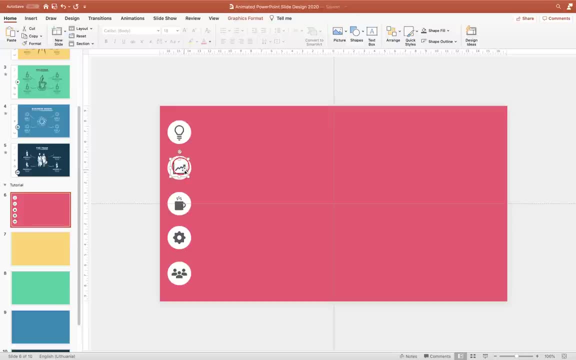 so i guess this is the same one. yep, all right, ladies and gentlemen, we are finished with these circles and the icons, so we can actually now insert a rectangle. so let's choose a rectangle tool and let's just draw a rectangle which covers all of our icons. let's send this rectangle to back. remove the. 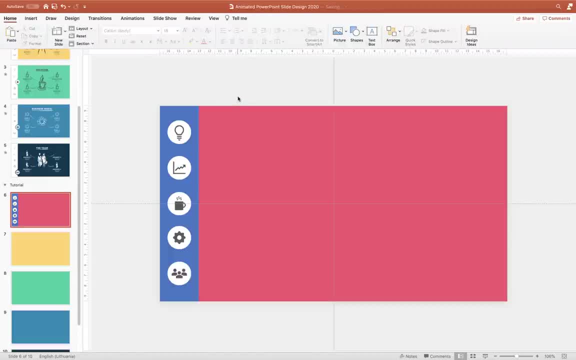 outline, all right, and we can see that we have a rectangle. and we can see that we have a rectangle and we can group all of these icons. hit command g or control g to group. let's make sure that everything is in the center. it is. that's awesome. so now we can ungroup all of these icons. 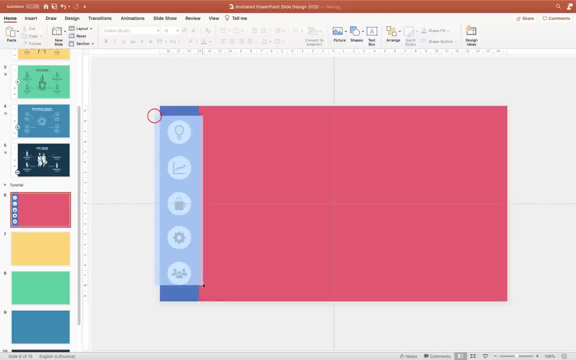 and now we can actually select all of these icons with the circles and let's just drag them here to the right side so that they touch, i mean to the left side, so that they touch the left side of the slide. but let's select the icons and bring them back. 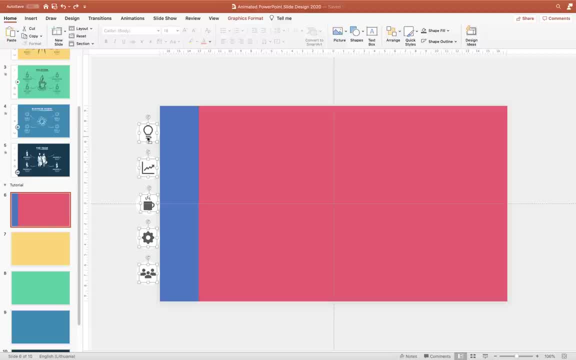 whoops, hold down the option or alt key to make a copy and bring back a copy, just like that. now let's make sure that the rectangle is white so that we can see what we're doing, just like that. and let's choose a different color for these icons. 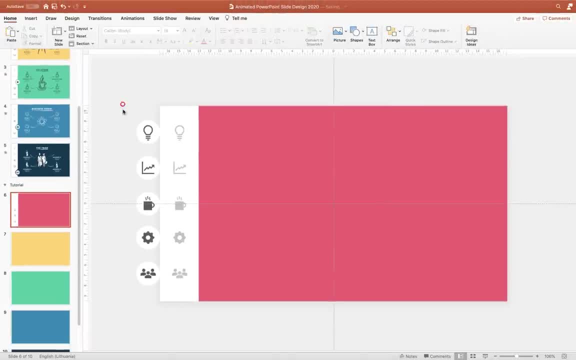 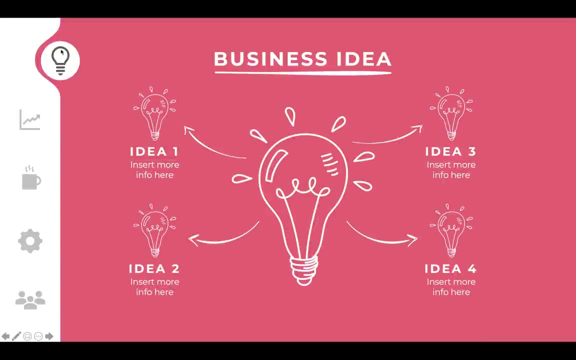 this one. so basically, here on the left side, we have the active colors or like these bubbles for the active icon status, and these are inactive. uh, you know icons. so, as you can see here here in the example, this one is active, so that's why we have this more. you know dark color and these have a slightly 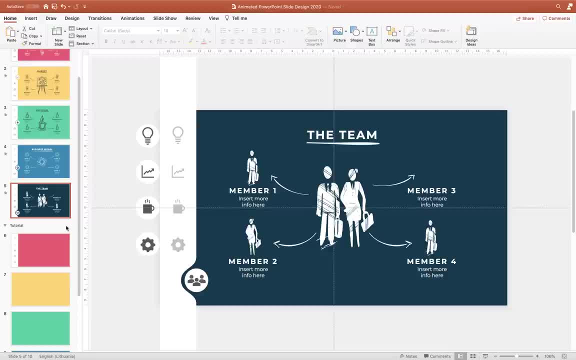 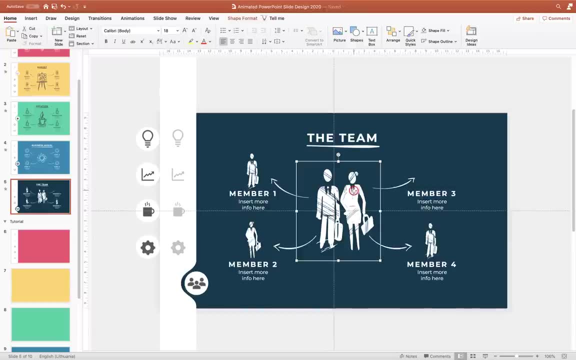 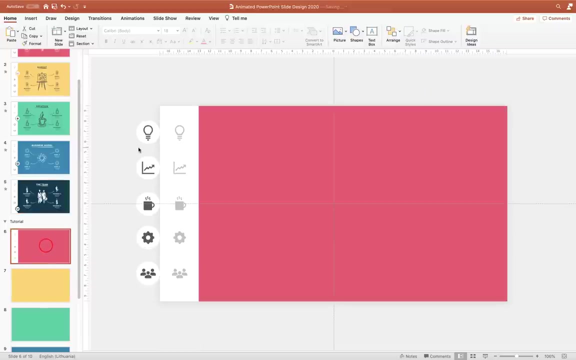 lighter color. so that's why we need a two copies, two copies of these um icons. somehow one team member is missing, so let's just drag a ladies, a lady somewhere right here. oops, hold down the option key to make a copy, just like that. awesome, all right. so now let's make sure that we group, group these guys together, so circle and icon. 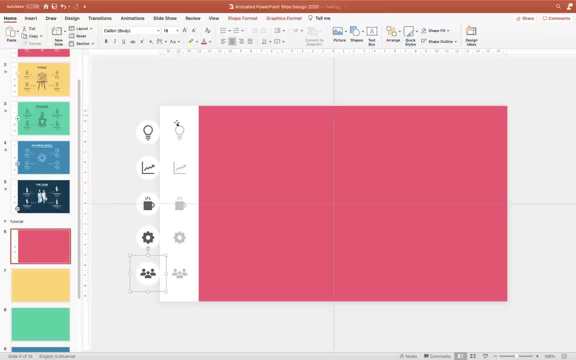 let's group them all right, and let's make sure that the biscuits are out there, so you can see that this ball got some sides and this fluted buttons. so that's why this is what we need right now: 10, all right, and let's make sure that all of these icons and this rectangle is in the front, bring. 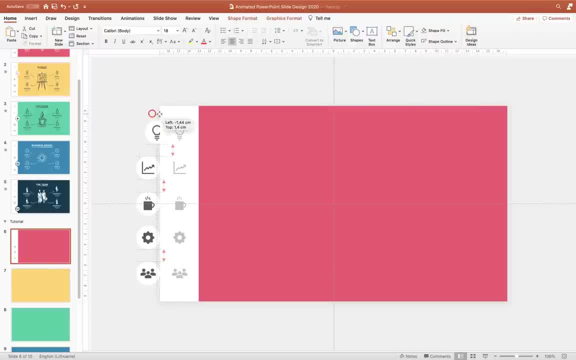 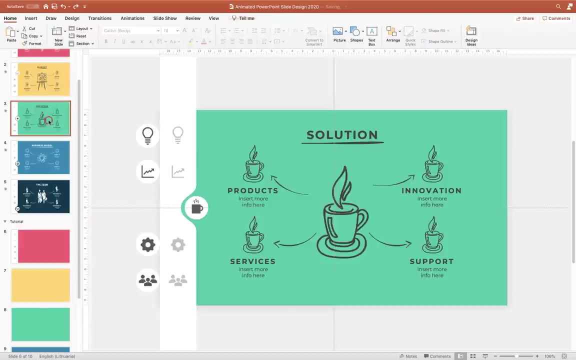 to front. okay, so that later on we will be animating this bubble and it should come, you know, below this white rectangle, just like that awesome. so now let's take care of the links, because, as you can see in this example, i have inserted the hyperlinks to each of these. 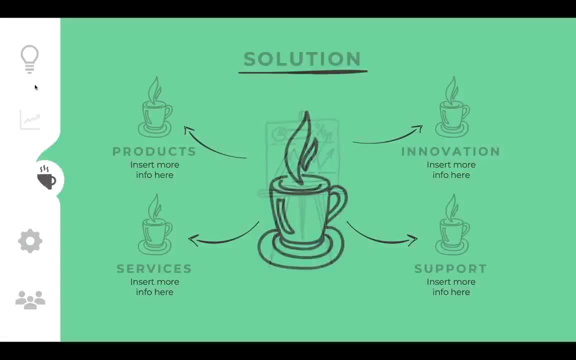 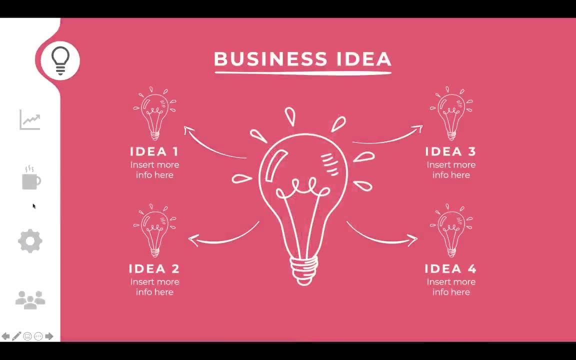 icons so you can use the arrow keys to navigate the presentation, but you can as well click on the icons and you can jump to any slide that you want, and to do that you need to insert links to these icons. so that's what we're going to do right now. 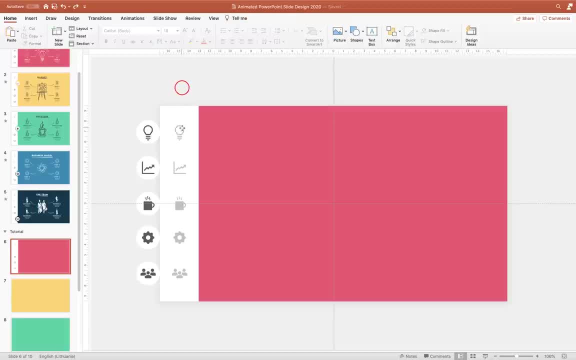 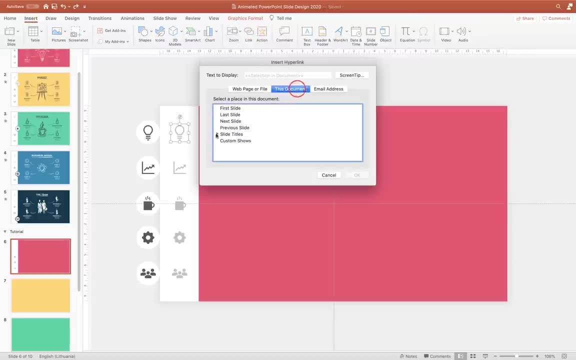 so for this first bubble icon, let's select it, go to insert, choose link and choose this document. slide titles, and in this case it is slide number six, so let's choose slide number six, for this next one is going to be slide number seven, and so on. so let me finish this up. 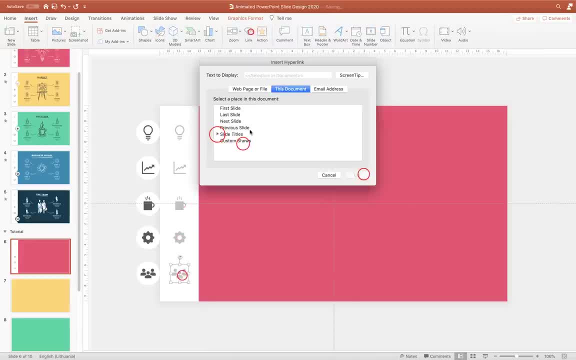 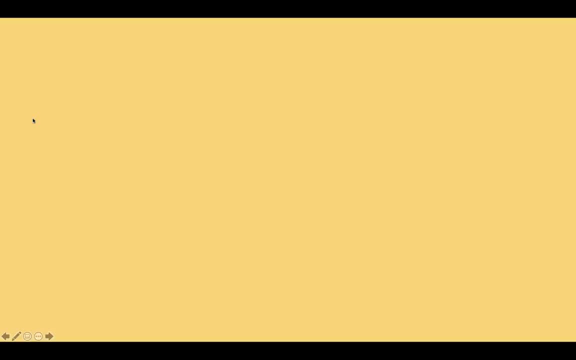 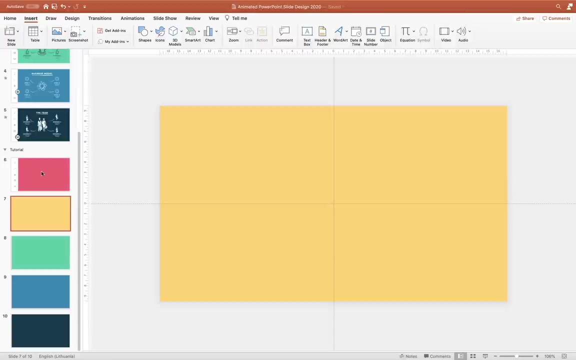 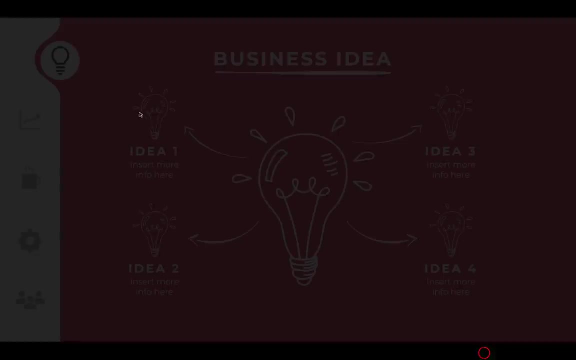 quickly, so now we can check it out on the full screen if our links are working. yes, they are working, but since the rest of our slides are empty, so there's nothing to see, okay, so now let me show you how we can actually create this beautiful, this beautiful cutout effect. as you can see, we have this. 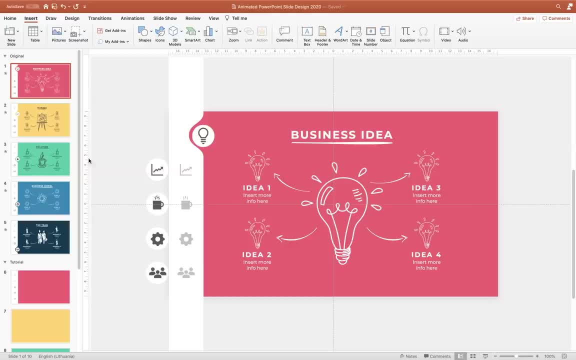 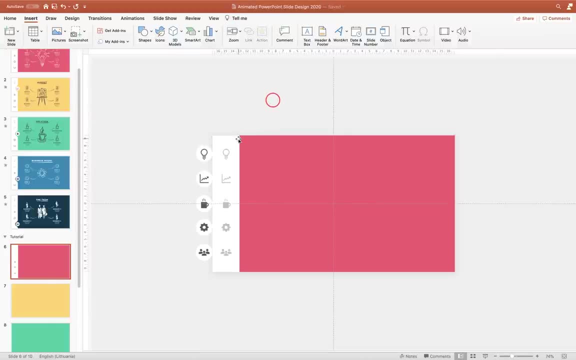 beautiful round cutout. so let's let me show you how it's done. and before we continue, let's actually zoom out a little bit and select this rectangle and hold down shift key and let's just drag it upwards like that. we need this rectangle to be bigger because 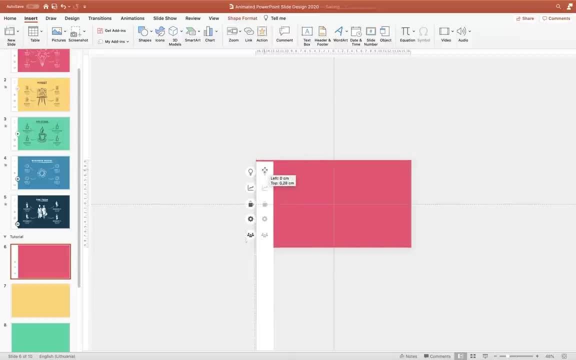 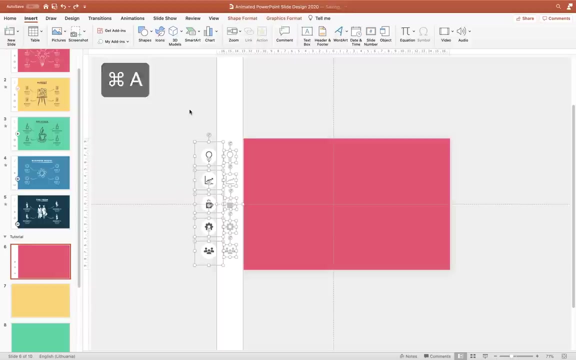 we'll be moving it up and down and we want this you know rectangle to cover the whole slide, so that's why we're making it extra long, just like that. all right, and now let's actually hit. command a, command a to select all of these objects. command a: 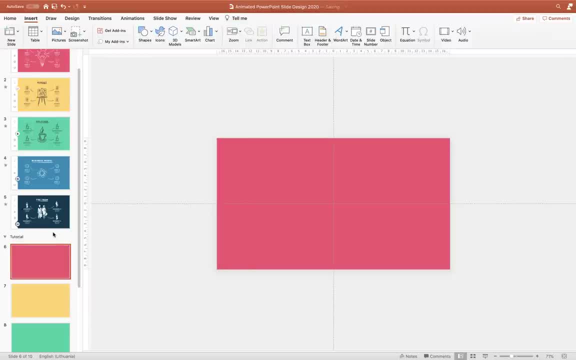 or ctrl a and hit command x to cut command a, and now we can go ahead and just run this up. so this we can unutrty simply running this full slide file. so let's just try it out as we go so we can cut all of these elements and let's paste them into slide number 8 command. 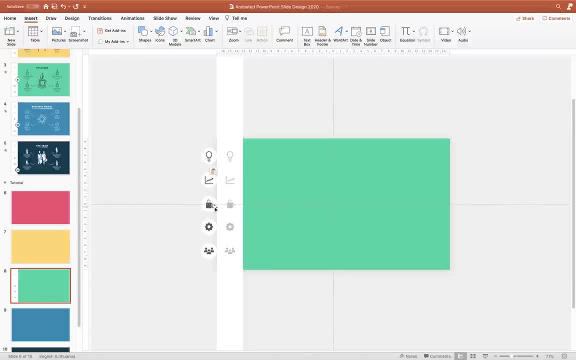 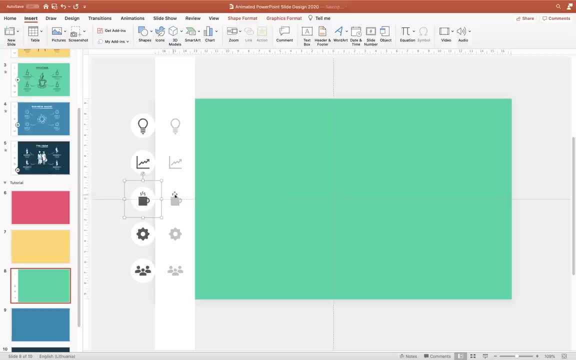 V or control V, because on this slide we can use this icon in the center to make the cutout. so let's actually move this icon to the center. we can change its color for a moment. let's just change its color to blue. all right, and now we? 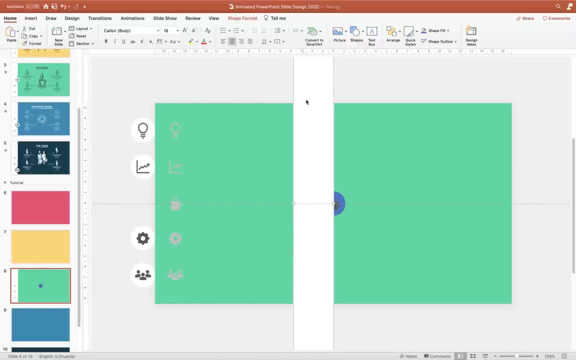 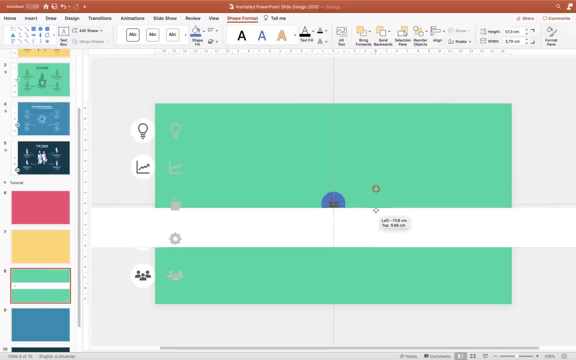 let's just drag this rectangle- the center as well, let's rotate it. rotate it to the right side, like this, and let's make sure we send it to back, and let's make sure it is aligned to the center, just like that. all right, so we have the. 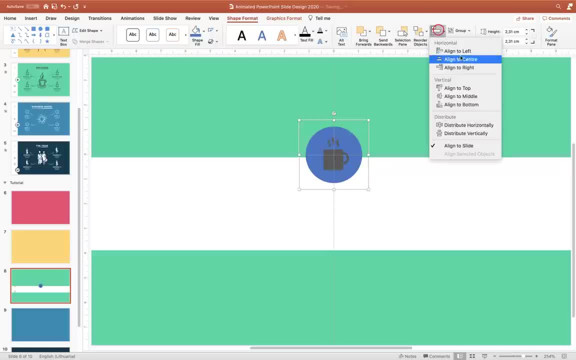 the cutout and now we can move this icon to the center, just like that. all right, so we have the this icon. let's just make sure it's in the center. it's really important all this icon. let's just make sure it's in the center. it's really important all. 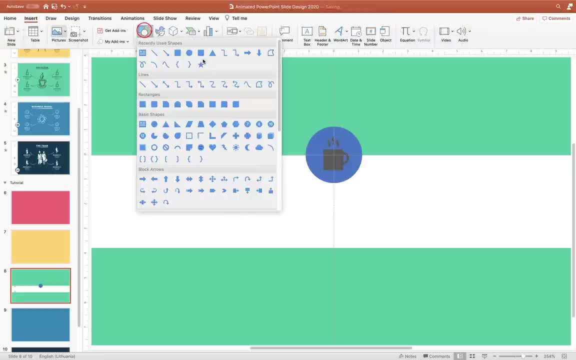 right. and now let's go to shapes and insert a triangle. hold down the shift right. and now let's go to shapes and insert a triangle. hold down the shift right. and now let's go to shapes and insert a triangle. hold down the shift key to get a perfect triangle. let's change. 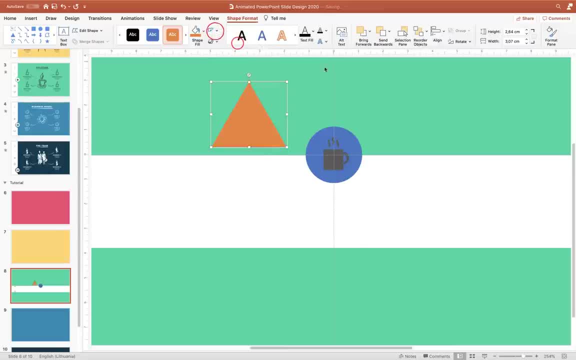 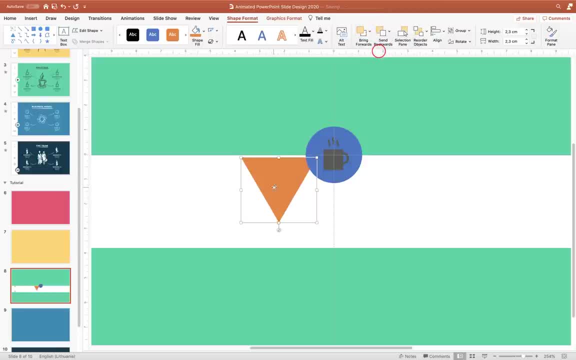 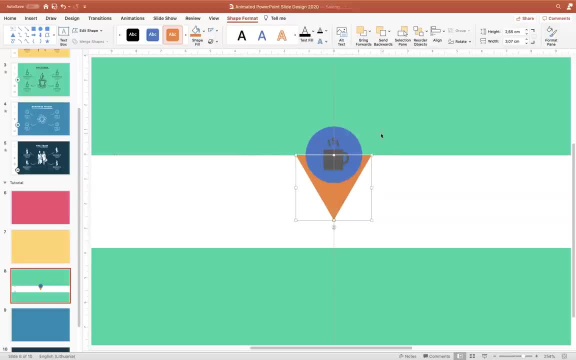 now let's place this rectangle in the. now let's place this rectangle in the center and like this to the top of this center and like this to the top of this center and like this to the top of this white rectangle, white rectangle, white rectangle, and now we can squish down this rectangle. 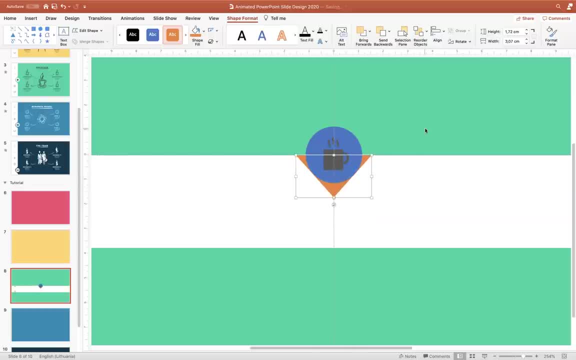 and now we can squish down this rectangle. and now we can squish down this rectangle. just like that, just like that, just like that again. let's align it to the top of this again. let's align it to the top of this again. let's align it to the top of this white track rectangle. 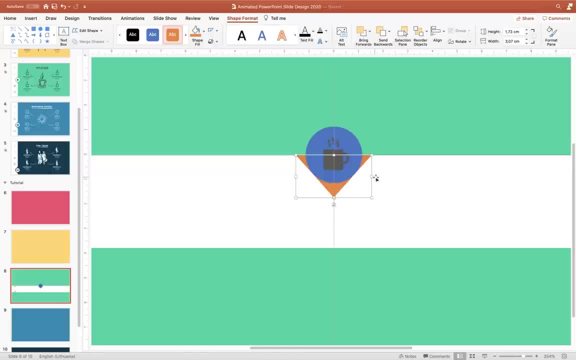 white track rectangle. white track rectangle. now, select the triangle and hold down. now select the triangle and hold down. now select the triangle and hold down the ctrl key, the ctrl key, the ctrl key, and this way we can make it wider. and this way we can make it wider. 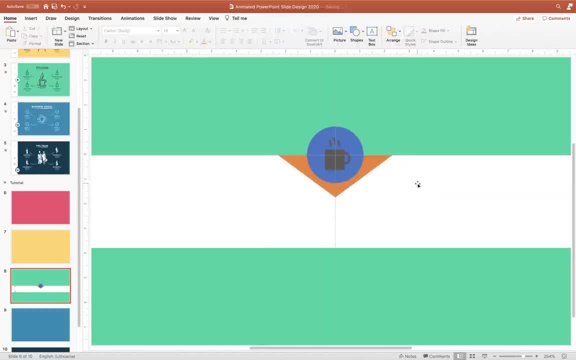 and this way we can make it wider. just like that, just like that. just like that, i think it's good enough, and now we can. i think it's good enough, and now we can. i think it's good enough, and now we can select, select. select the white rectangle, hold down the shift. 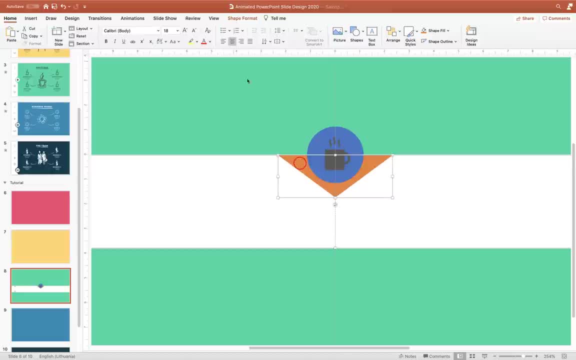 the white rectangle hold down the shift. the white rectangle hold down the shift. key select. key select. key select the triangle now go to shape format. the triangle now go to shape format. the triangle now go to shape format. merge shapes and choose subtract. merge shapes and choose subtract. 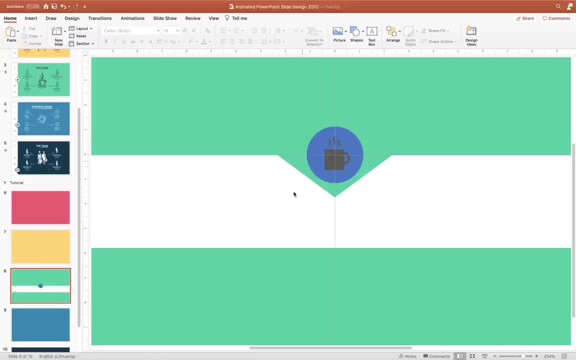 merge shapes and choose, subtract. this way we have subtracted the triangle. this way. we have subtracted the triangle this way. we have subtracted the triangle from the rectangle, from the rectangle, from the triangle. color once again. so it looks color once again. so it looks color once again. so it looks beautiful. 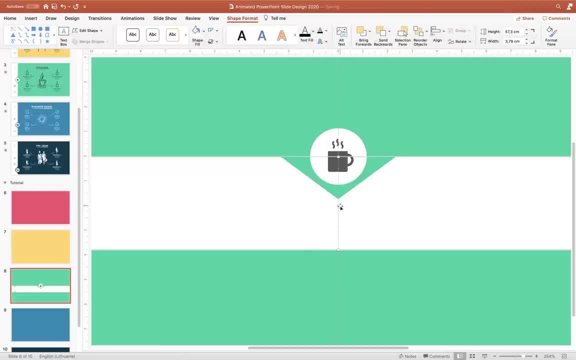 beautiful, beautiful. all right, and now we can select this. all right, and now we can select this. all right, and now we can select this rectangle shape and choose edit points. rectangle shape and choose edit points. rectangle shape and choose edit points. and now we will have to play with these. 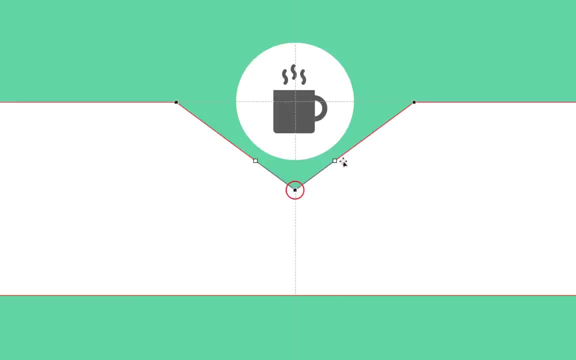 and now we will have to play with these, and now we will have to play with these points a little bit. so let's just click points a little bit. so let's just click points a little bit. so let's just click on this, on this, on this bottom point, we're getting these white. 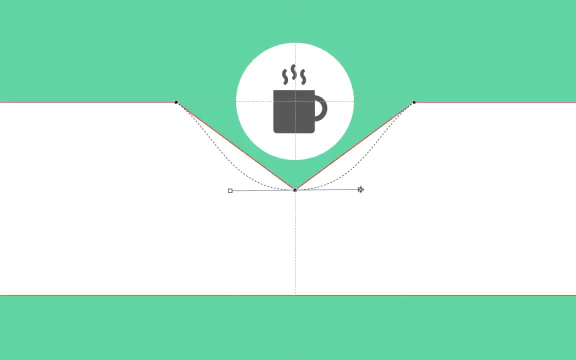 bottom point. we're getting these white bottom point. we're getting these white handles, handles, handles. so just hold down the shift key and so just hold down the shift key and so just hold down the shift key and drag them down like that, and it's whoops once again. 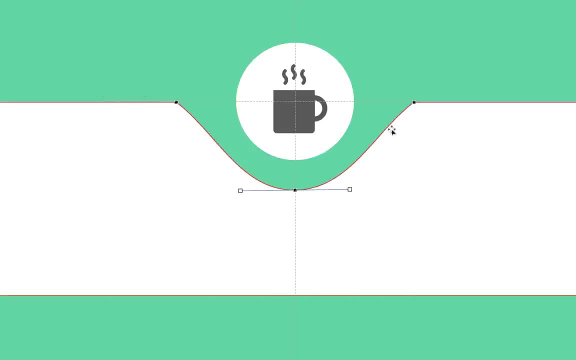 and it's whoops once again, and it's whoops once again. and, as you can see, we're getting this and, as you can see, we're getting this and, as you can see, we're getting this: nice, uh, beautiful curve, nice, uh, beautiful curve, nice, uh, beautiful curve. and for these points as well, we can. 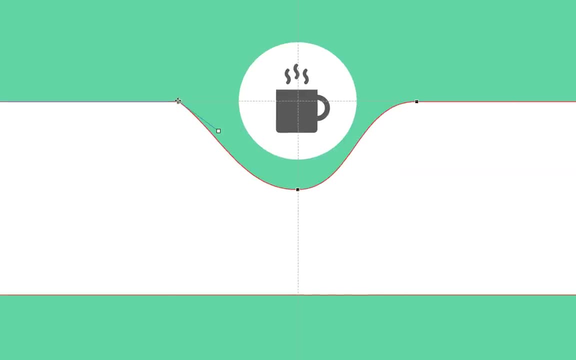 and for these points as well, we can, and for these points as well, we can drag this handle just like that, drag this handle just like that. drag this handle just like that. for this one as well, let's make it. for this one as well, let's make it. 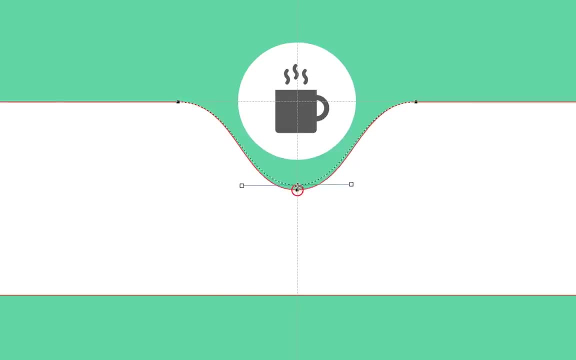 for this one as well. let's make it something like this, something like this, something like this: we can bring up this point and we can. we can bring up this point and we can. we can bring up this point and we can drag these handles outwards slightly. 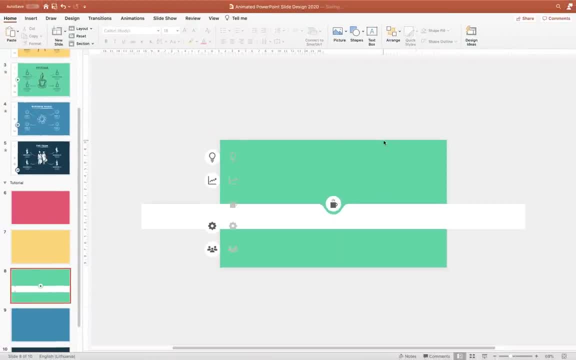 drag these handles outwards slightly, drag these handles outwards slightly, and i think it looks pretty good. and i think it looks pretty good, and i think it looks pretty good, all right, so all we have to do right now. all right, so all we have to do right now. 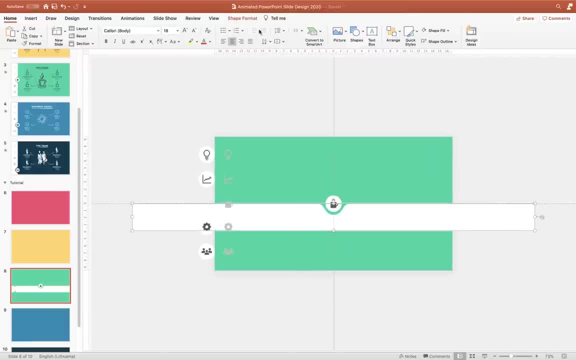 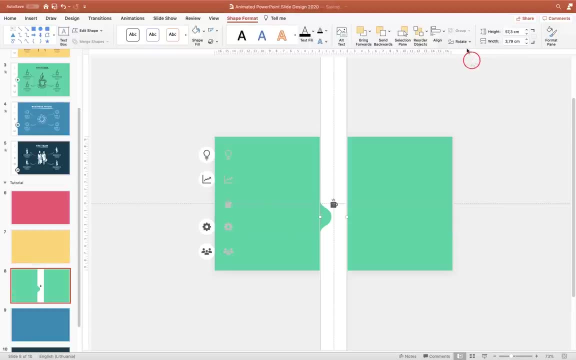 all right. so all we have to do right now is just put back everything into place. is just put back everything into place, is just put back everything into place. so, so, so, let's flip this rectangle to rectangle to rectangle, to the left side, the left side, the left side or to the right side, just like that. 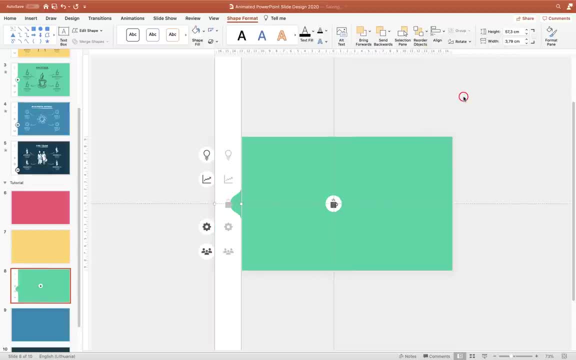 or to the right side, just like that, or to the right side, just like that. let's align it to the left side, and let's align it to the left side, and let's align it to the left side and let's align it to the middle, so it's in. 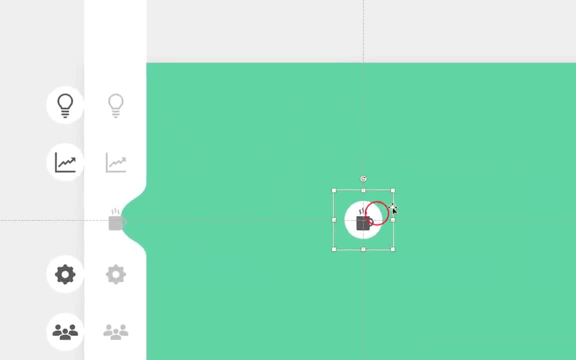 let's align it to the middle, so it's in. let's align it to the middle, so it's in the middle, the middle, the middle. that's beautiful, that's beautiful, that's beautiful. now, let's just bring this circle to now. let's just bring this circle to. 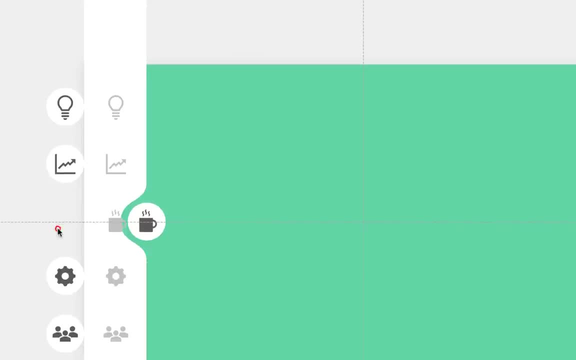 now let's just bring this circle to this position, this position, this position, okay, and for this inactive icon, let's go to: and for this inactive icon, let's go to. and for this inactive icon, let's go to graphic format and choose no, fill it's graphic format and choose no, fill it's. 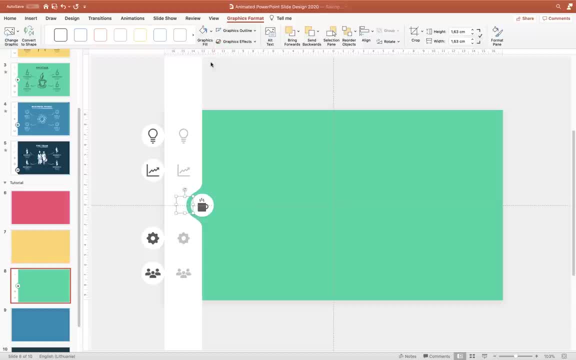 graphic format and choose no fill. it's really important, really important, really important. to make a this icon to have no fill. to make a this icon to have no fill. to make a this icon to have no fill. that's that's how it works. that's that's how it works. 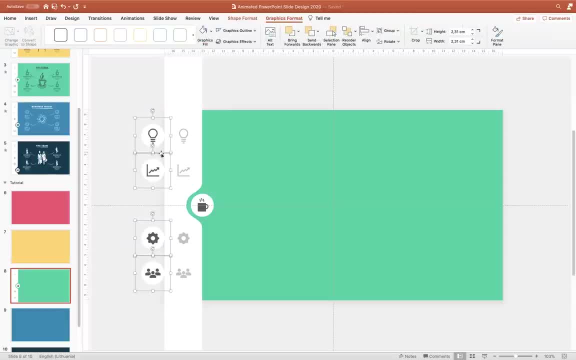 that's, that's how it works, okay, and once again, let's select all of okay. and once again, let's select all of okay. and once again, let's select all of these, these, these bubble icons, and this one as well, hold bubble icons, and this one as well, hold. 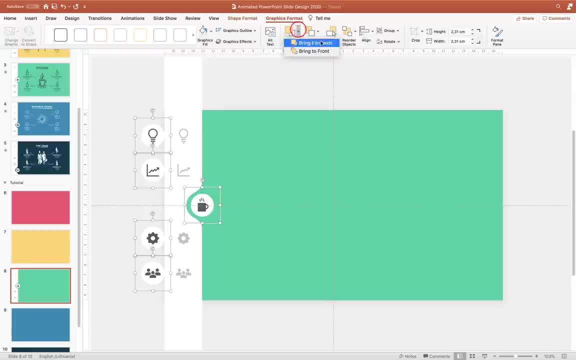 bubble icons, and this one as well, hold down the shift key to select it and down the shift key to select it and down the shift key to select it, and let's make sure we send them. let's make sure we send them, let's make sure we send them to back. 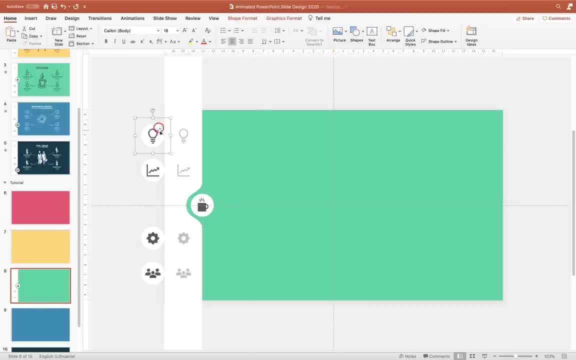 to back to back so that, so that, so that this rectangle and all of these icons, this rectangle and all of these icons, this rectangle and all of these icons are in the front, are in the front, are in the front. that's awesome, that's important. that's awesome, that's important. 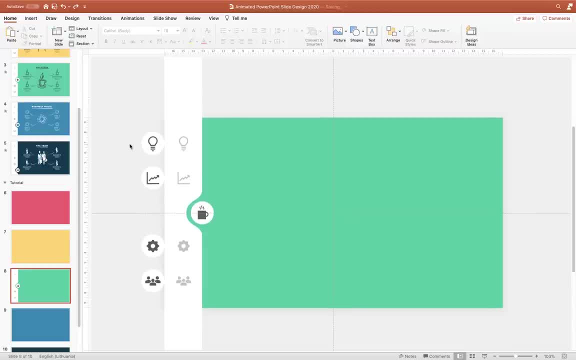 that's awesome, that's important. all right, so we're pretty much uh all right, so we're pretty much uh all right. so we're pretty much uh finished with you know creating all of finished, with you know creating all of finished, with you know creating all of the elements that we need. so now we go. 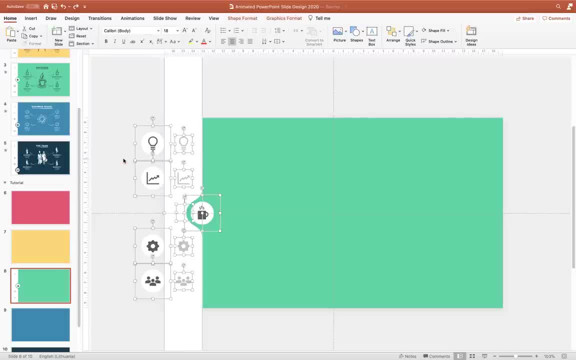 the elements that we need. so now we go, the elements that we need. so now we go to the fun part, to the fun part, to the fun part. so let's select all of these uh elements. so let's select all of these uh elements. so let's select all of these uh elements. hit command c or control c to copy. 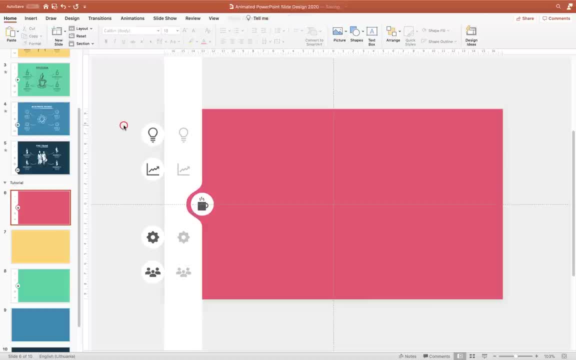 hit command c or control c to copy. hit command c or control c to copy. and now let's paste them right here. and now let's paste them right here. and now let's paste them right here into slide number six, into slide number six, into slide number six. all right, so now let's just select this. 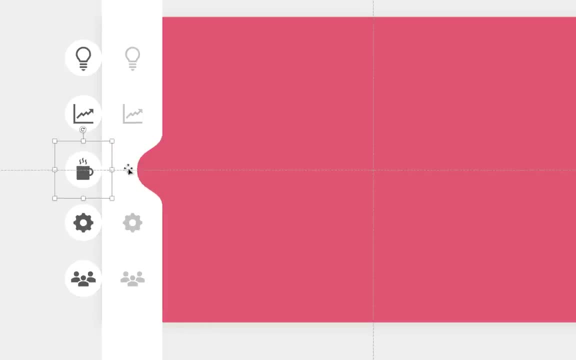 all right, so now let's just select this. all right, so now let's just select this. bubble icon, let's move it right here. bubble icon, let's move it right here. bubble icon, let's move it right here. and for this guy, let's turn back the. 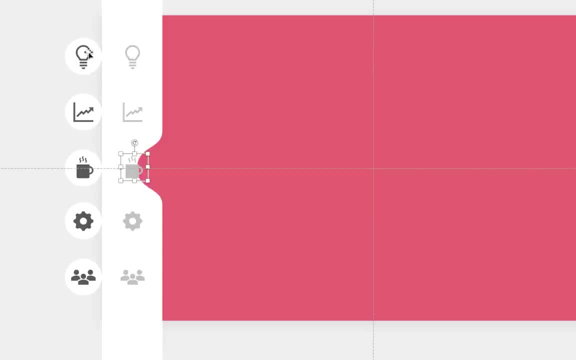 and for this guy, let's turn back the. and for this guy, let's turn back the color of this guy. color of this guy, color of this guy. all right, and now grab this. all right, and now grab this. all right, and now grab this bubble icon. let's move it here. 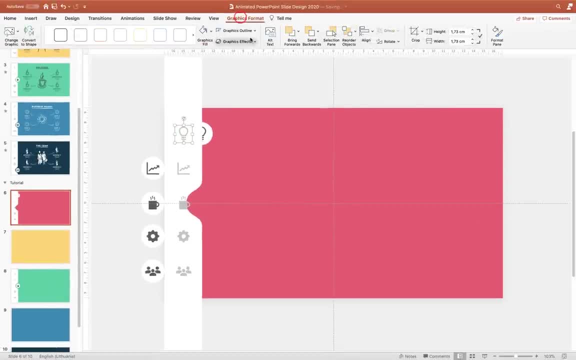 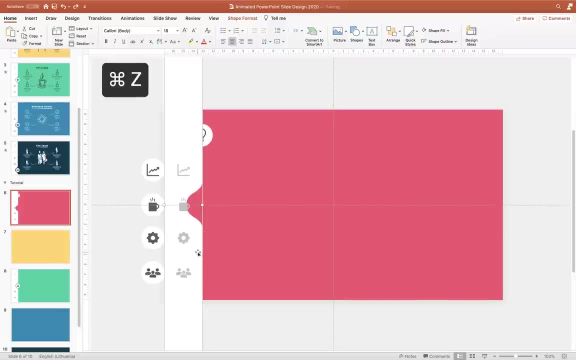 bubble icon, let's move it here. bubble icon, let's move it here. let's make, let's make, let's make this icon: no, fill all right. no, fill all right. no, fill all right now. let's select this rectangle now. let's select this rectangle now. let's select this rectangle and. 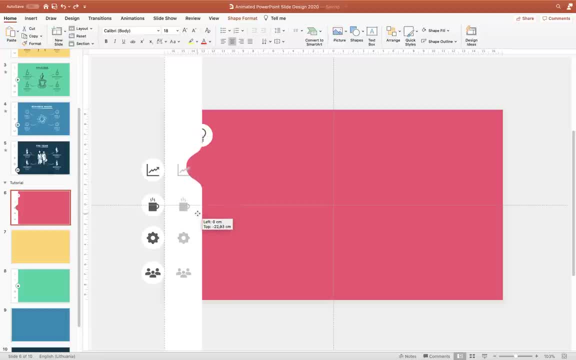 and and let's move it upwards. you can hold down- let's move it upwards. you can hold down the shift key so that you know you move in a straight line and position it like this, okay, so, uh, now we can select all of the slides, from slide number six to slide number 10. 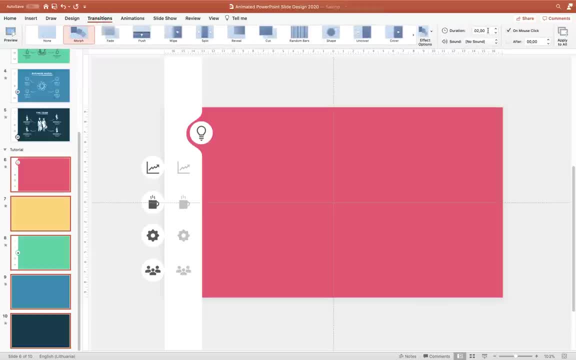 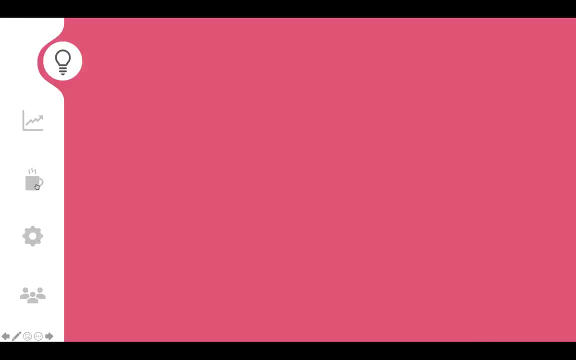 go to transitions, make sure you select morph and we can make it faster. 0.5 seconds, all right, and we can basically check it out if it, if it's working, okay, so we can click on this icon and we can click back to the first one. so yeah, it's looking beautiful and, of course, the rest. 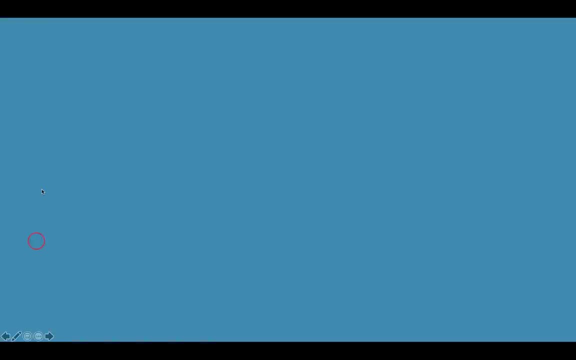 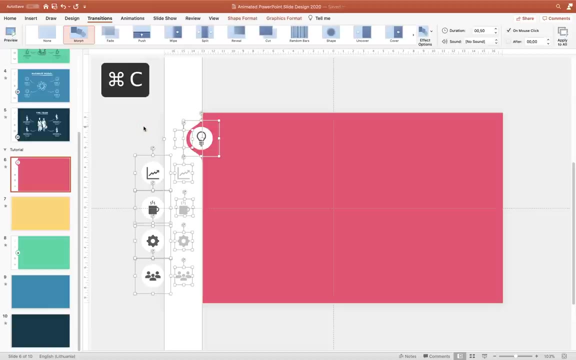 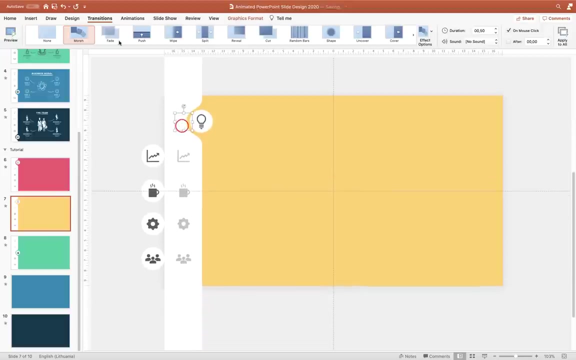 of the icons. we haven't done them yet, so it's empty. so let's continue with that. so let's just hit command a to select everything and let's paste everything into slide number seven, all right? so in this case, let's bring the visibility of this icon. 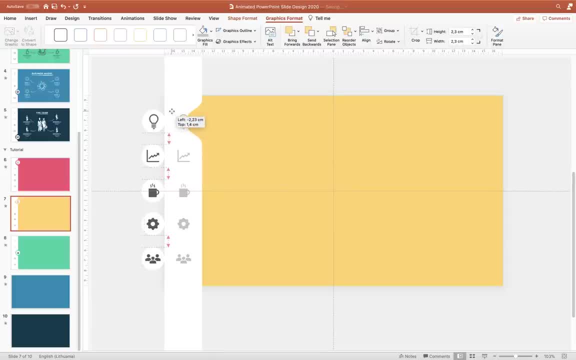 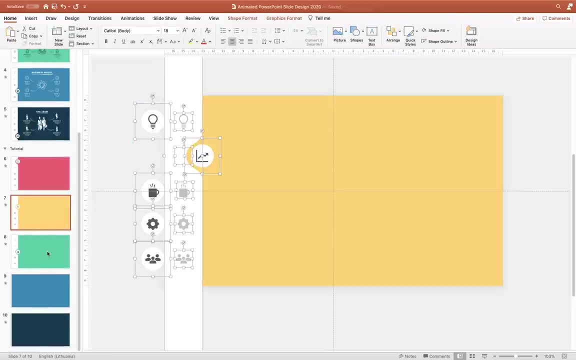 let's bring this guy to the left side, let's bring this guy to the right side. always you can hold down the shift key- and for this guy, let's make it unvisible, invisible, and let's bring down the rectangle. and this is pretty much the same steps that i'm going to repeat, for 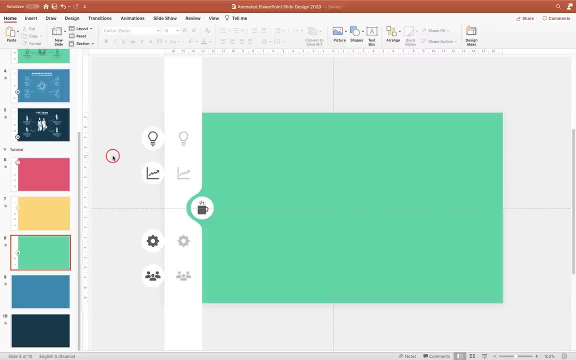 the. for the rest of the slides, we can actually copy all of the elements from the slide number eight and paste them to slide number nine. all right, so let's uh place this one to the left side. let's un, uh, let's make this. uh, we can just copy the color from this. 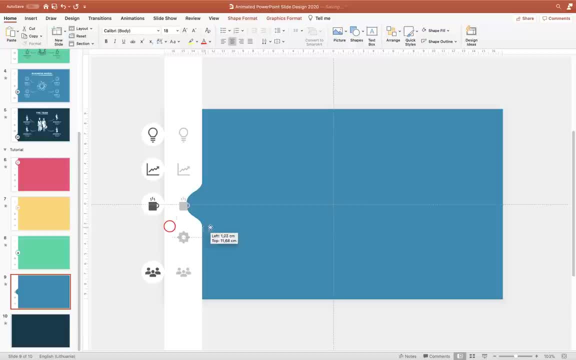 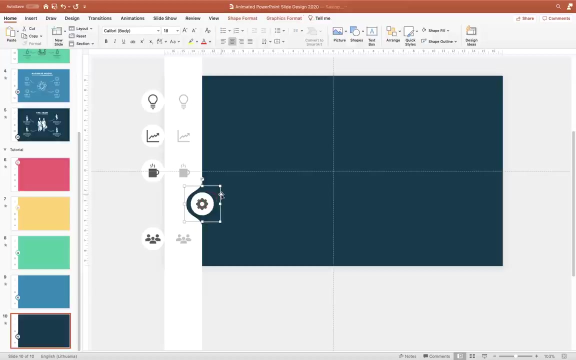 icon. all right, now let's bring this bubble icon to the right side. this one gets invisibility powers. that's awesome. and we bring down the rectangle. it's beautiful. once again command a or control a to select everything, and hit command c to copy paste everything into the last slide and once again bring this guy to the left side. 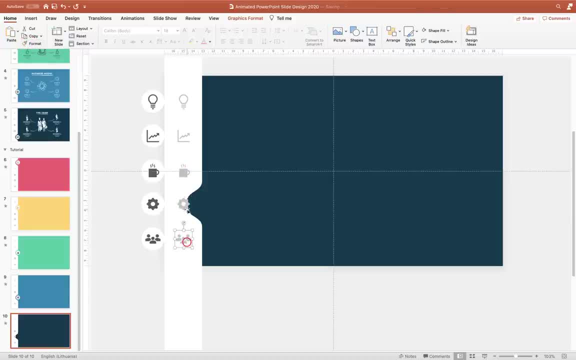 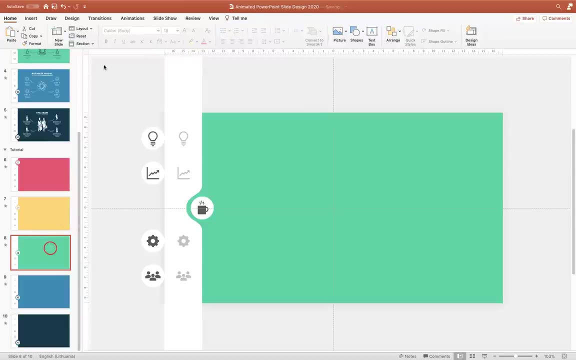 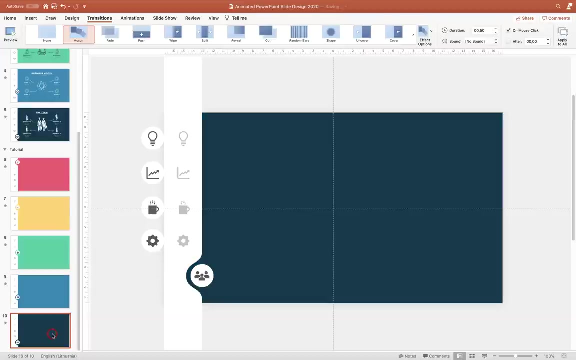 let's copy this beautiful color, this icon, this one becomes invisible and this guy goes to the right side, and then the rectangle goes here and, as you can see, all of these slides have, uh, morph transition, and morph transition really helps with making all of these animations, all right. so now everything should be working, just 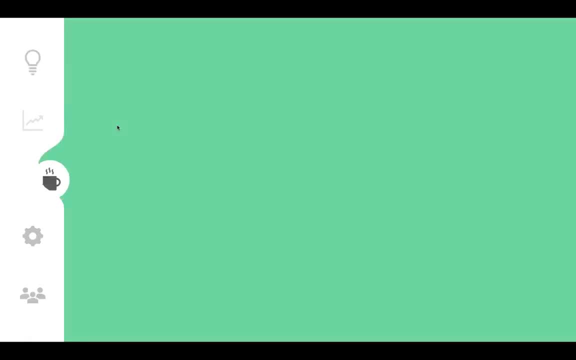 perfectly and we can test it out by using the arrow keys left and right and as well. you can click on any of these icons and you can jump straight to the last slide or straight to the first slide. that's super duper awesome and, by the way, if you are viewing your presentation on a tablet,